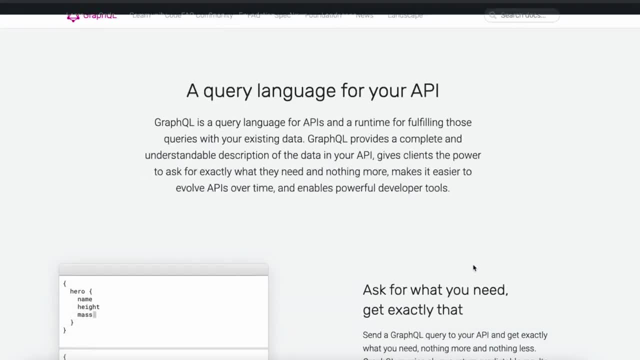 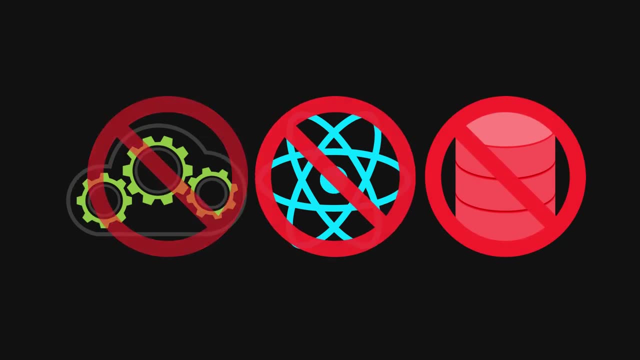 familiar with GraphQL. you might be familiar with GraphQL as a query language that describes an API request. The important distinction that a lot of beginners don't understand is the fact that GraphQL isn't a technology library or a database, but rather it is actually a query language. that 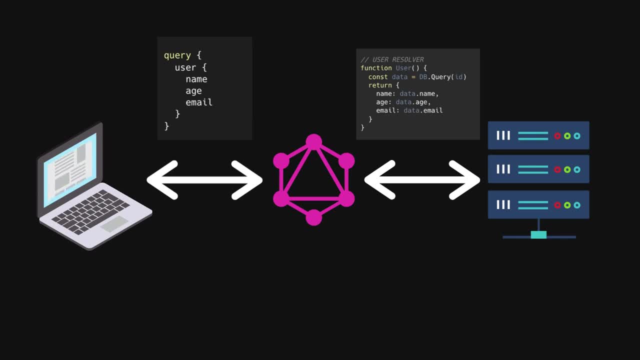 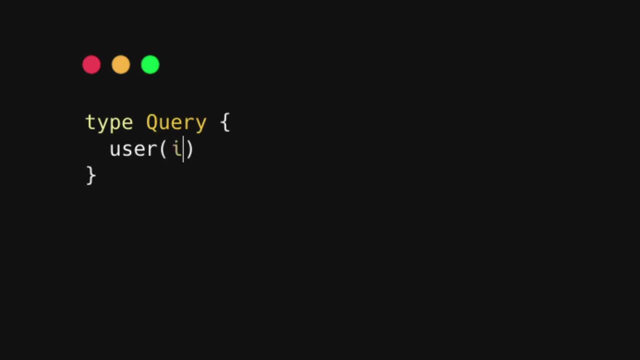 exists as a layer between your frontend and your backend allowing you to expose the data that you sent from your server to your client in the format described by a GraphQL API. So the frontend will always be communicating with GraphQL and the backend will always also be communicating with. 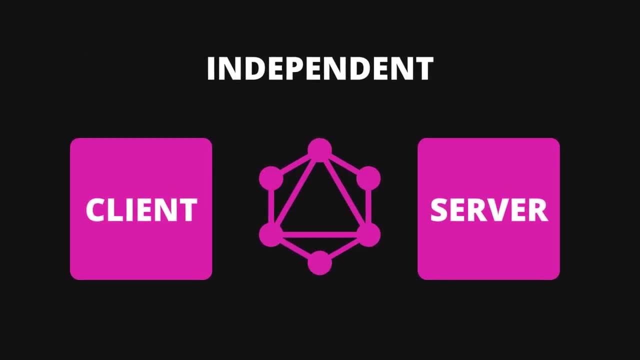 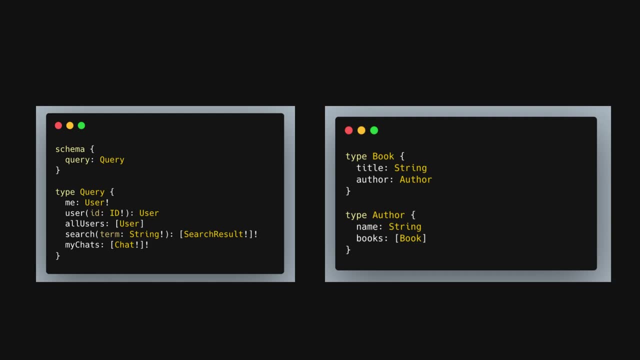 GraphQL, making it so that the frontend doesn't really need to know a lot about the backend and the backend doesn't really need to know a lot about the frontend, And the thing that connects both of them is the GraphQL API that sets a certain standard for what kind of data it accepts. 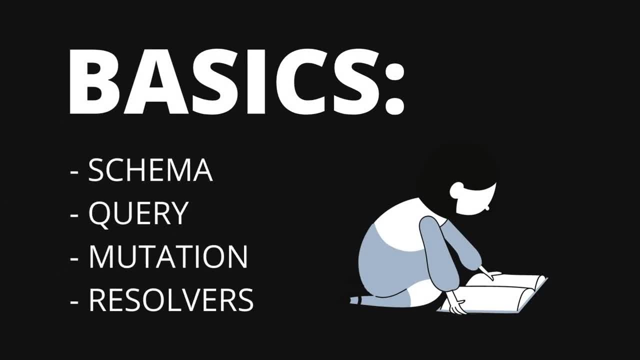 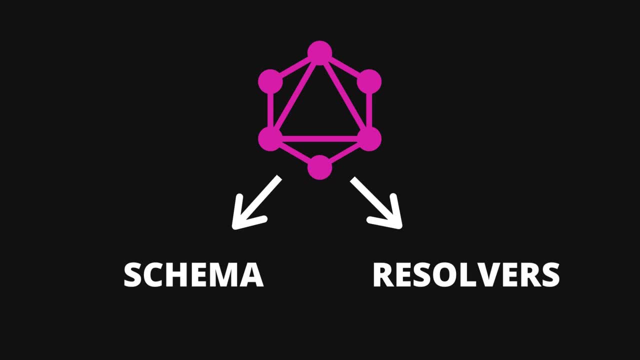 Now I know a lot of that is kind of confusing because it was very confusing for me when I started learning GraphQL. However, in this video I want to go over a little bit of the basics of GraphQL, by first of all explaining what exactly is a GraphQL API? So a GraphQL API? 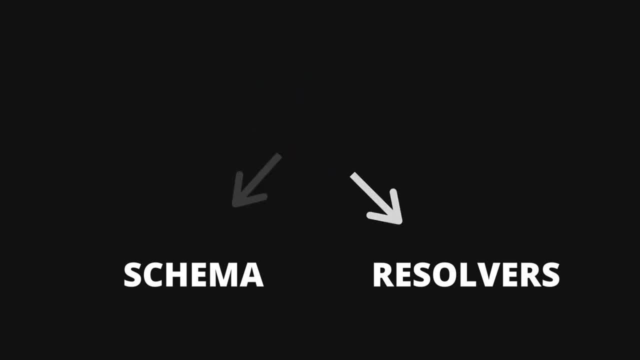 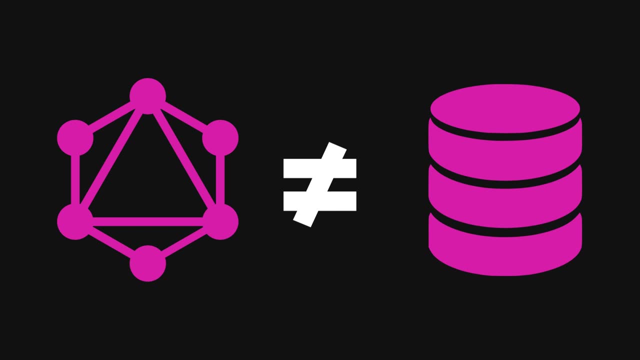 is usually divided into its schema and its resolvers. The schema is not the same as a database schema that you might have heard in the past, because GraphQL is completely independent from your database. The schema is basically a way to describe how your API will work. 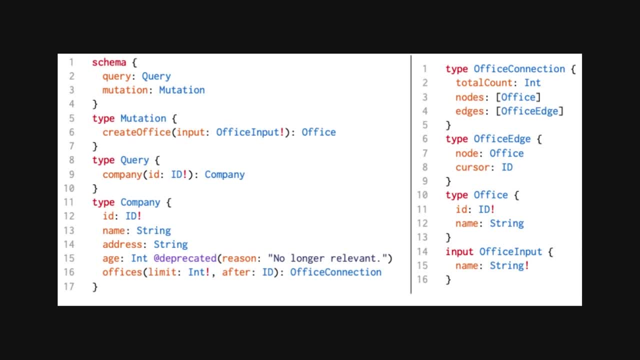 including what kind of data it will receive, what kind of data it will send and what kind of data it will mutate. This is where you will describe all of the types that you will create in your GraphQL API. So, for example, if you want to have users. 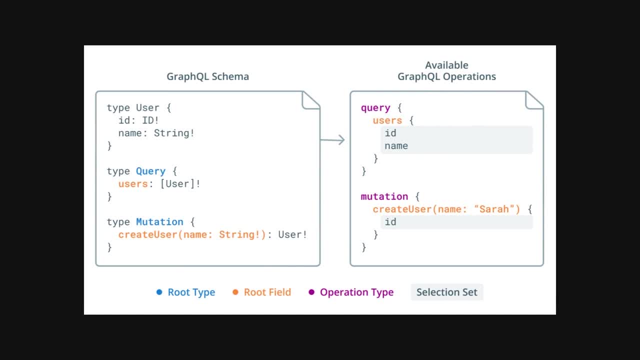 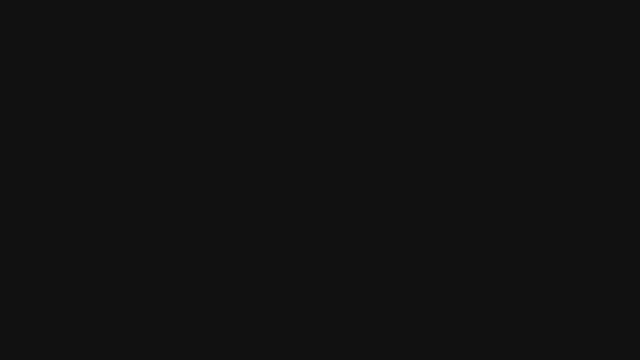 in your website and you want the GraphQL API to add users, delete users, change users, however you want. you need to create a type called user and put it inside of your schema. Every schema has two required types: the query and the mutation type. The query type is used. 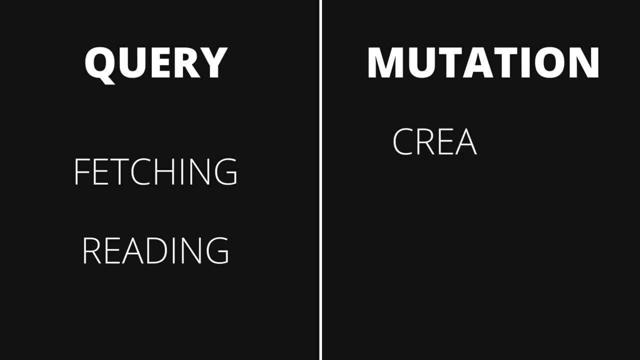 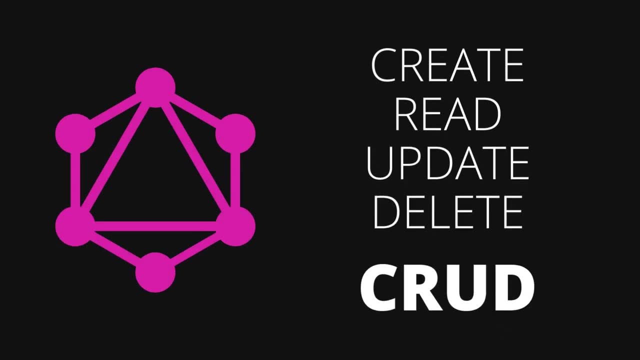 for fetching and reading data from your API, while the mutation type is used for creating, updating or deleting data from your API. When a schema has both, it allows CRUD operations in your app In order to get an idea of how this works. 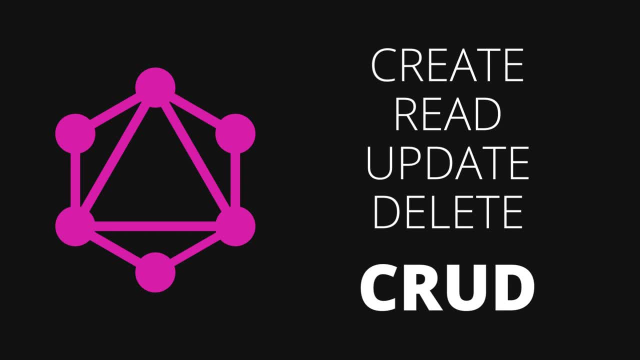 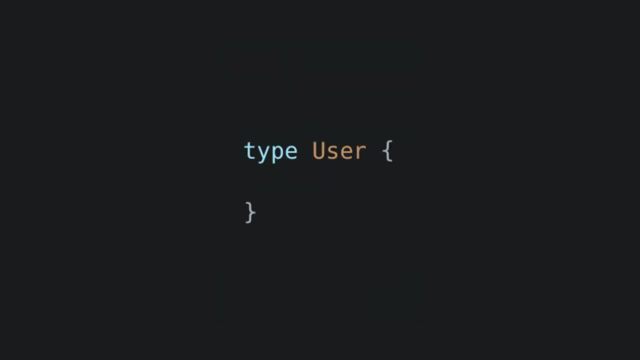 let's create a GraphQL API that reads and mutates data related to a user. First we have to write the schema and create the query and mutation types. Then we create the user type that we're going to use For each type. we can add fields with different types related to the user. 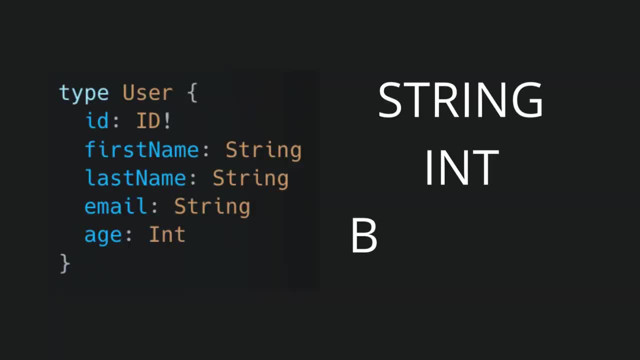 GraphQL has some basic types like a string, an int, a boolean and many others. But if we wanted to create a new type and nest it inside of another type, we can. For example, let's create another type called job, And that type will include: 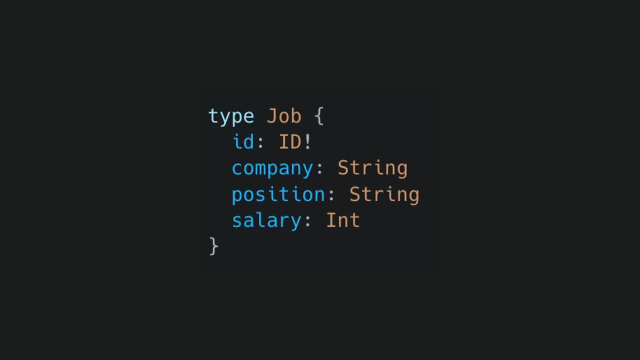 information about, for example, the job name of the user, the position and the salary. Now if we want to create a field in each user where we specify what job they have, we can just set the return type for the field to be job And that will tell GraphQL that when you 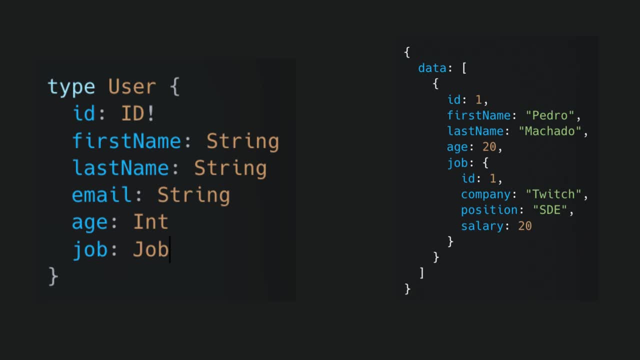 ask for a user's job, it should return all of the information related to the job type. The reason why we describe all of this in this way is so GraphQL can be very strict with the format of the data it handles. We can even make some fields. 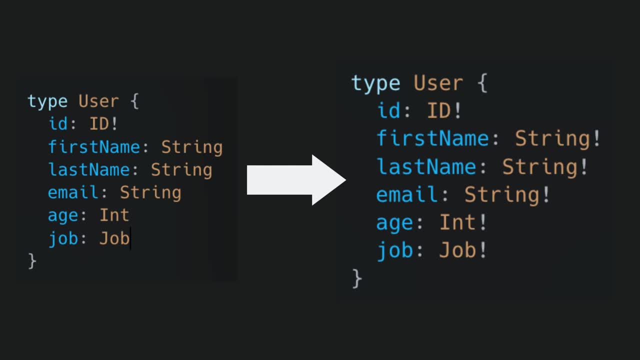 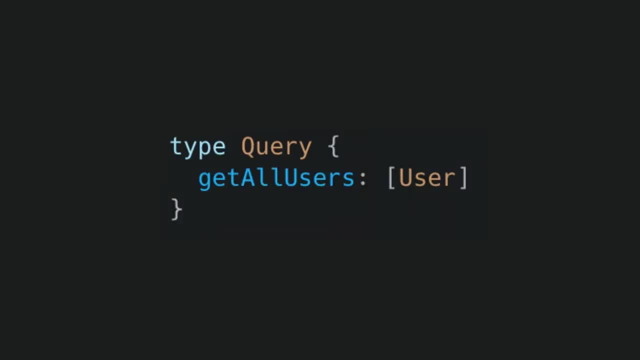 required, if we want to, by adding an explanation point at the end of the return type. Now that we have the actual type for the user, let's just add a query field to our query type. Our first query will return a list of all users. We can do this by giving it a name such as get all users and. 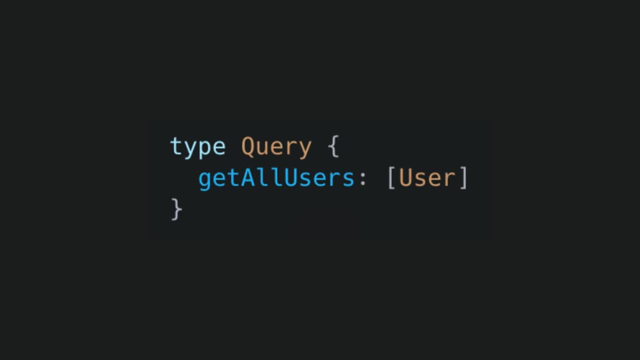 setting the return type to be a list of users by adding a little square bracket around the type. We can also make a simpler query which basically just fetches an individual user, But to do that we do need the ID of a user, because that's how you usually do it with an API. So we'll have to pass. 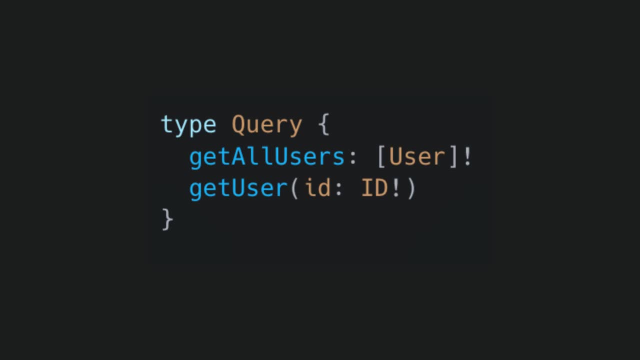 in an argument to this query and say that for this query, we also need to get the ID from the front end, And this it's a very important functionality in GraphQL and you do it this way. Now to create some mutations, we can just do something very similar. For example, let's go back to our 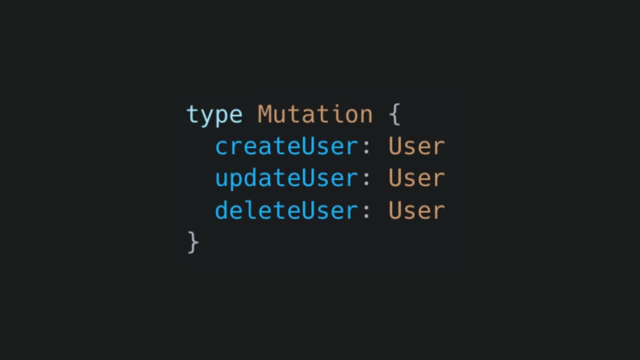 database. Let's create three different types of mutations. that allows us to create, update and delete a user. Each field will require a different piece of information to execute properly. For example, to create a user, we need information about the user sent from the front end to then.